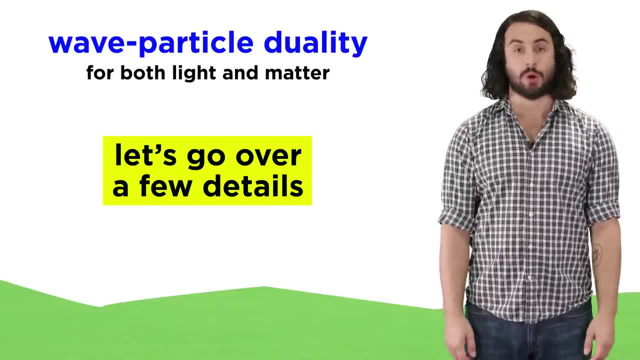 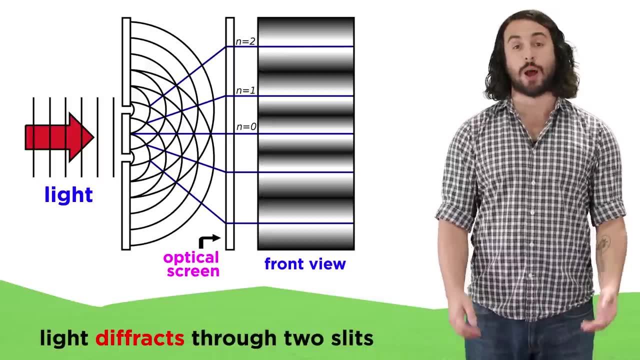 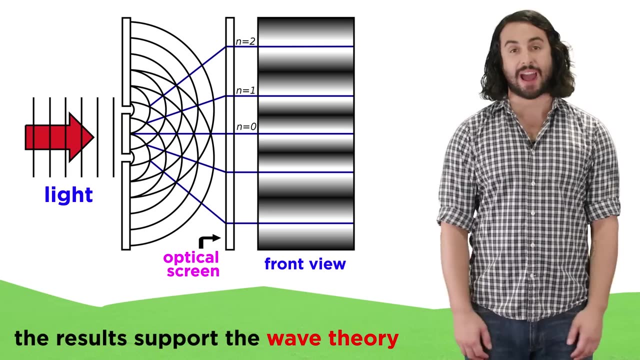 But we glossed over some of the technical details, so let's zoom in for a moment. In 1801,, Thomas Young performed experiments where light was passed through a plane with two slits in it, striking a screen beyond The diffraction and interference patterns that resulted clearly supported the wave model. 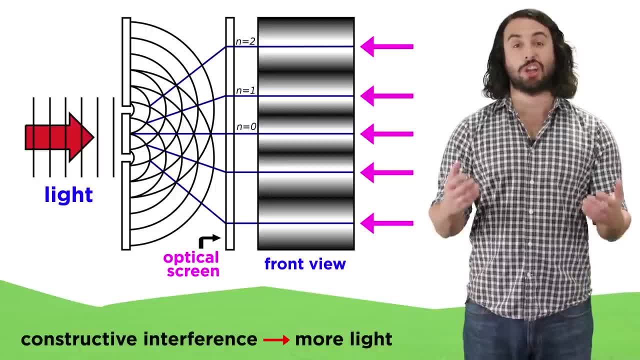 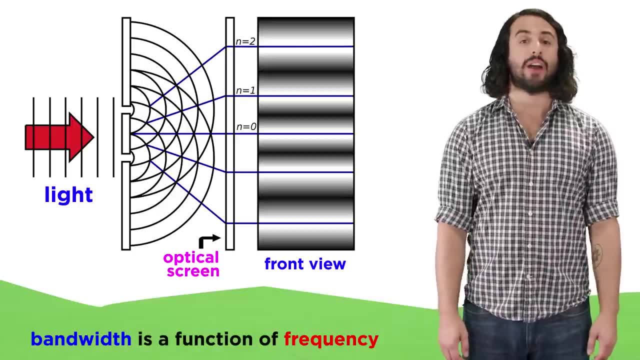 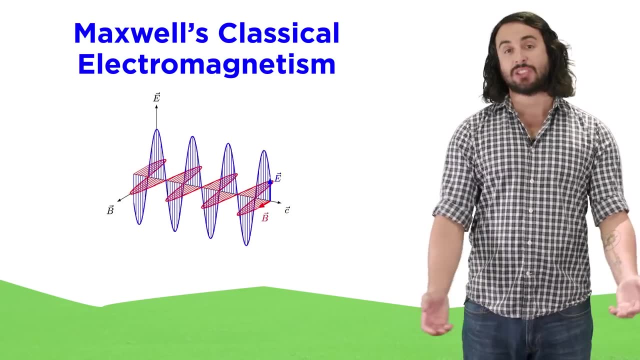 of light, with the brighter bands representing constructive interference and the darker bands representing destructive interference, With the width of the bands being a function of the frequency of the light. Later in the century, Maxwell showed that light is a wave of oscillating electric and. 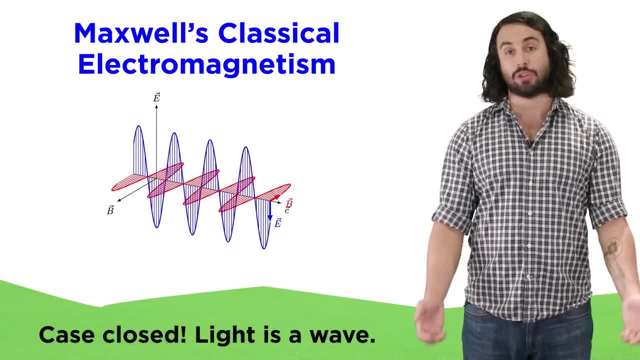 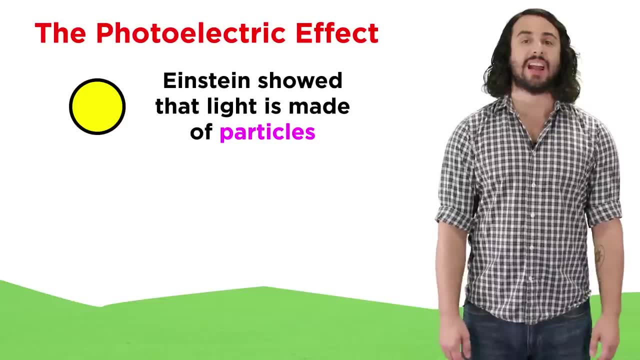 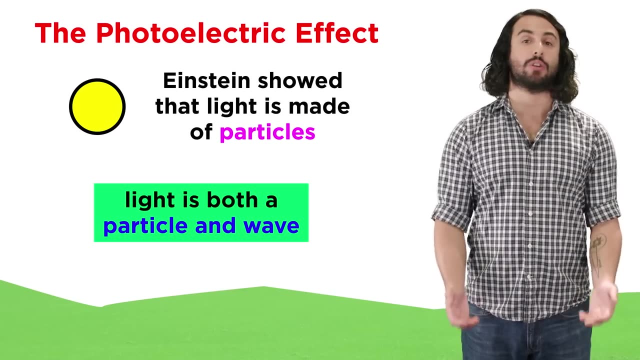 magnetic fields. so it seemed as though the case was closed on the declaration of light as waves. But as we said, in 1905, Einstein solved the problem of the photoelectric effect by assigning particle nature to light. Thus wave-particle duality was born. 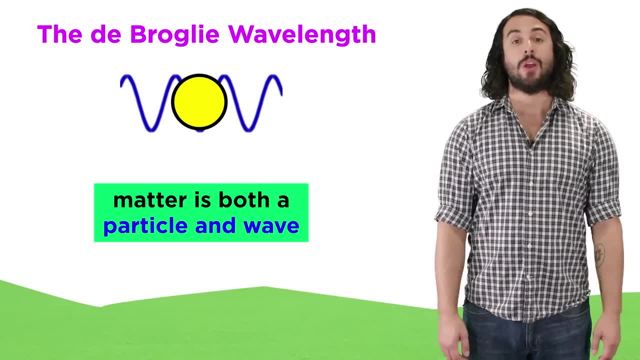 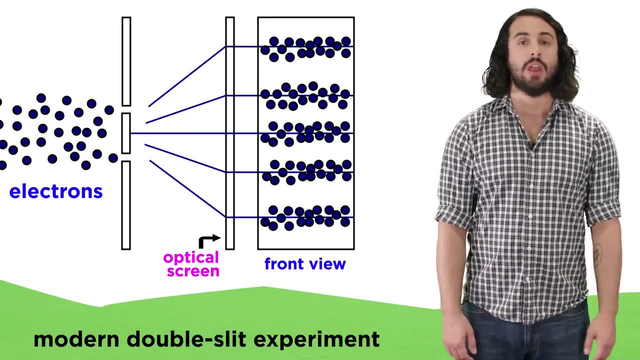 Later, de Broglie proposed that particles must therefore also display wave-like behavior, and this was shown to be true in an experiment just like Young's more than a hundred years prior. This modern version is what we are typically referring to when we talk about the double-slit. 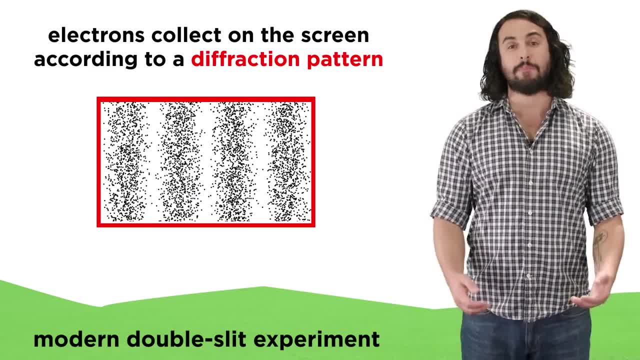 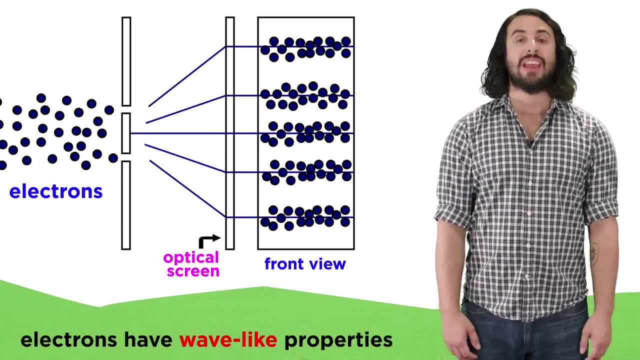 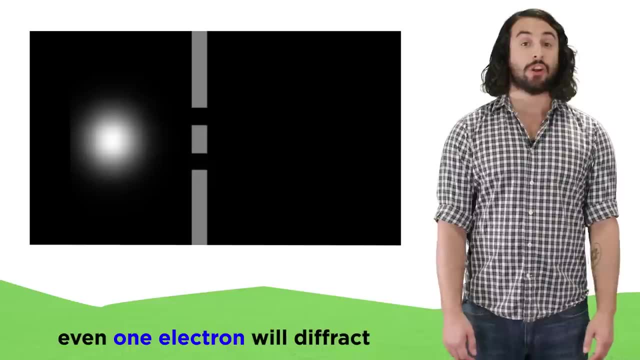 experiment. From this it was shown that a beam of electrons exhibits diffraction and interference patterns just like light does. This demonstrates the wave-like properties of electrons and, by extension, matter in general. Later low-intensity experiments showed that even an individual electron, when passing, 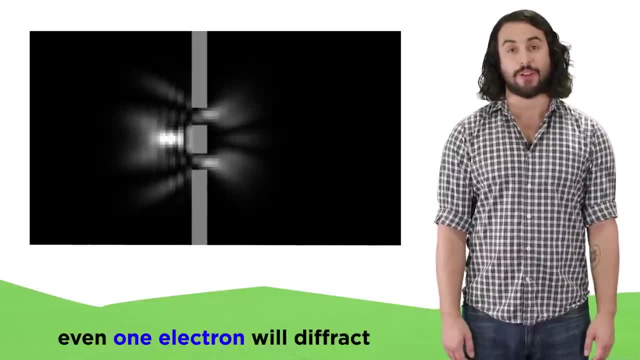 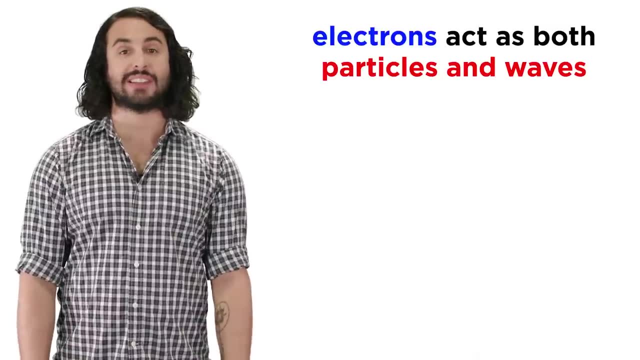 through biprisms or slits will interfere with itself, making the wave-like nature of the electron undeniable. So it was shown that electrons act as both particles and waves. but not just electrons: neutrons were also shown to exhibit diffraction patterns. 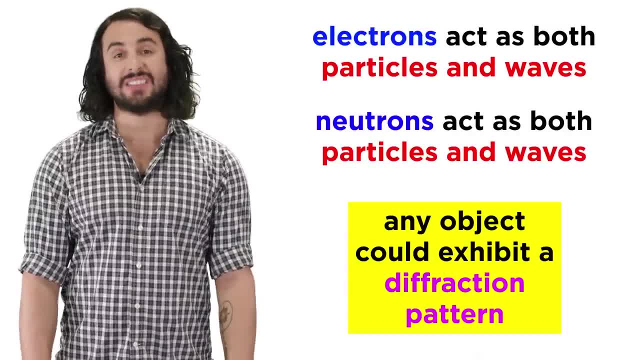 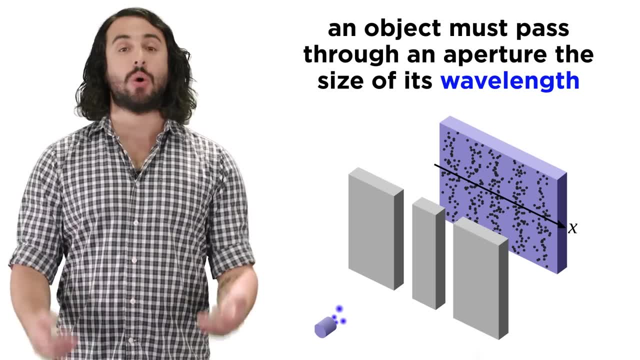 So it was shown that electrons act as both particles and waves. but not just electrons: neutrons were also shown to exhibit diffraction patterns. It must be understood that, since all particles are also waves, literally any object could hypothetically exhibit a diffraction pattern, so long as the object passes through an aperture.